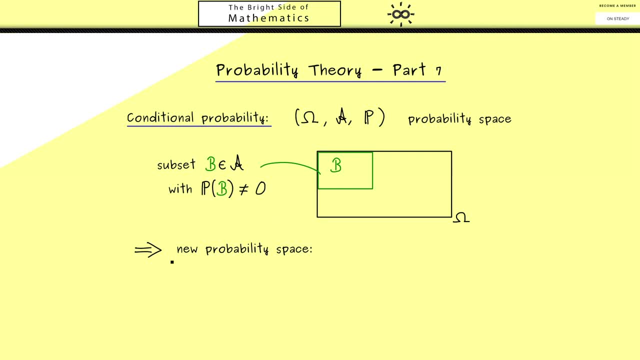 probability measure. Moreover, we even get a whole new probability space. Now, instead of omega, we take b as the new sample space. Of course, we can simply do that, but then we have the question: what is the new sigma algebra and what is the new probability measure For the? 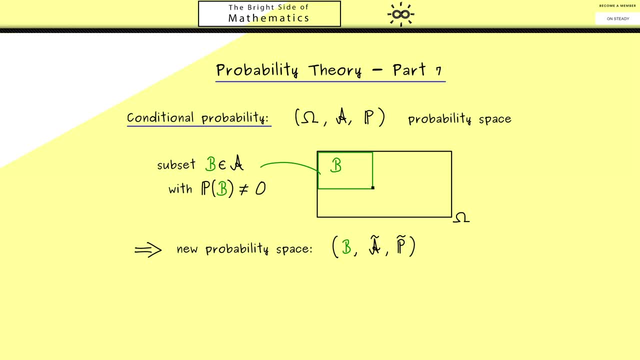 sigma algebra. the answer is very straightforward. If we only want to work in b, we can only consider subsets of b. So we can take any element a from the original sigma algebra if it fulfills that a is a subset of b, And then of course we could measure the probability of a as 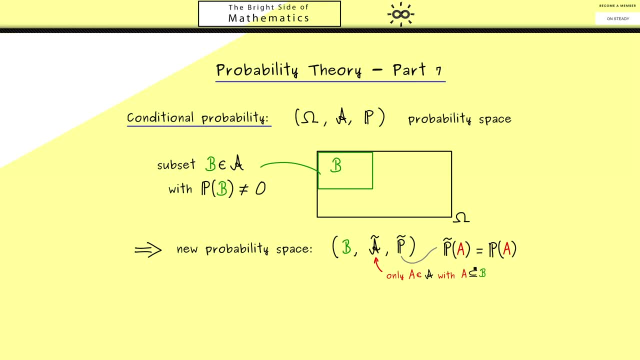 before. Therefore, p tilde could simply be the same probability measure as before. So in our picture it would just give us the area of the set a. However, there we see a problem, because the maximal area we would get out would be the area of b, which is in general not 1.. 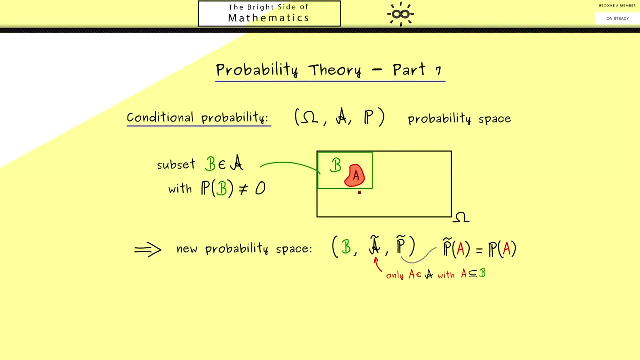 Indeed, what we rather want would be a ratio, So the ratio of the area of a to the area of b. Hence in our formula we have that p a gets divided by p b. Only now we have a well defined probability measure. Because now, when we put in 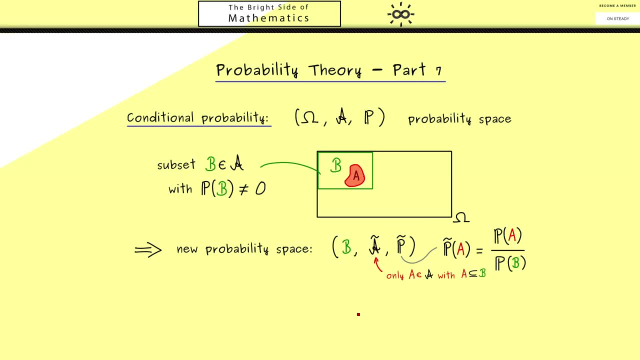 the sample space b, we get out 1.. Ok, now i can tell you this is almost a full idea of a conditional probability. I say almost because actually we don't want to change the sample space and the sigma algebra. In other words, this means that we also have to consider sets a that are not subsets. 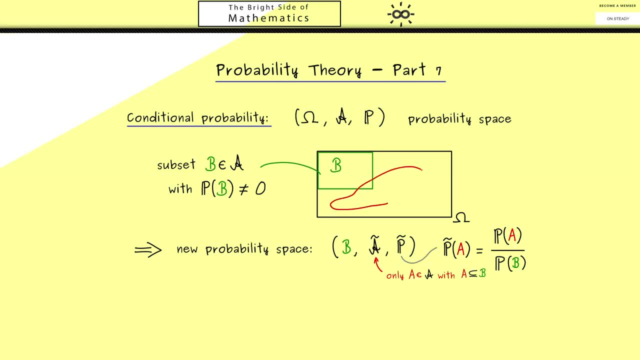 of b, For example, they could look like this. So, as you can see, it could have a very large area, but the intersection with the set b could be small. Therefore, you might already know how we can transform this definition here to the whole space omega. So our new probability space only gets a new probability measure. 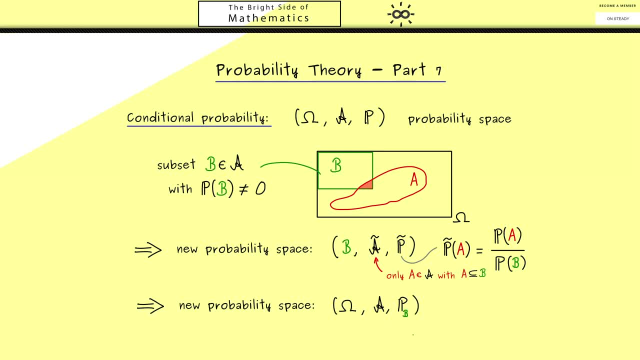 And for the moment, let's put an index b to it. Now for the definition. please remind yourself that we still want to measure the ratio of two areas, Which means the denominator is the same as before, Which means the whole area of b, But the numerator now should be this area. Speaking of 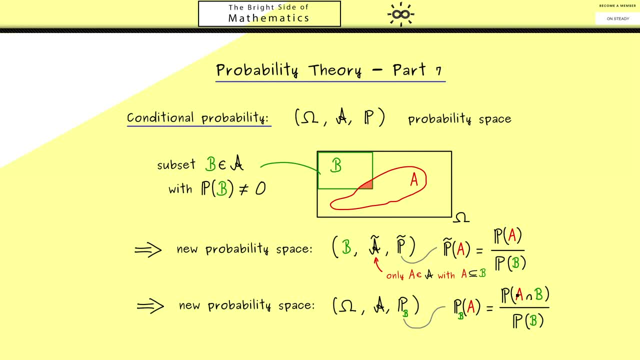 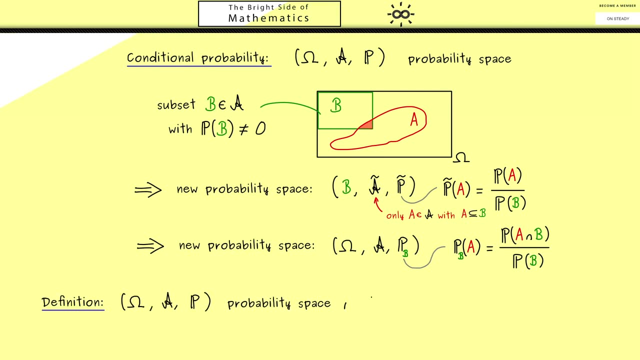 probabilities. this would be the probability of the intersection, And now this is the definition of the conditional probability of an event a under the event b. Therefore, i would suggest putting this into a formal definition. Of course, the assumptions are the same as before. We have a probability space and also a set b with a non-zero probability, And then we can. 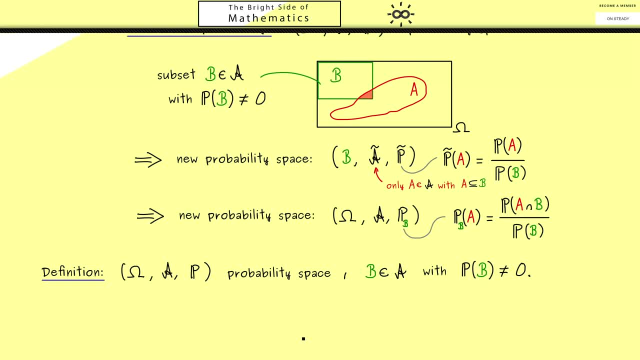 define the conditional probability as a new probability measure. In fact, sometimes this index notation is used for this probability measure, but often we have another notation, Namely one uses the bar inside the parentheses and puts the condition, the set b, to the right hand side, And then we call this number the conditional probability of the event a under the condition b. 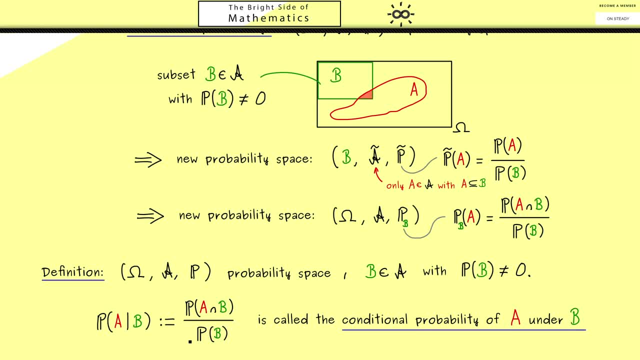 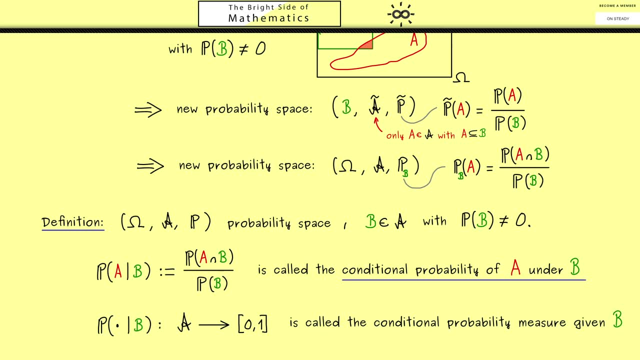 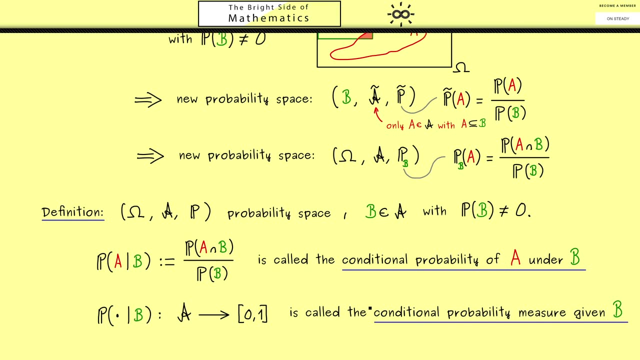 Moreover, if one wants to talk about the abstract probability measure, one uses the following notation: We simply put a dot where the set should go in, And then we call this well defined measure the conditional probability measure given b. Ok, then, please never forget, this measure has an. 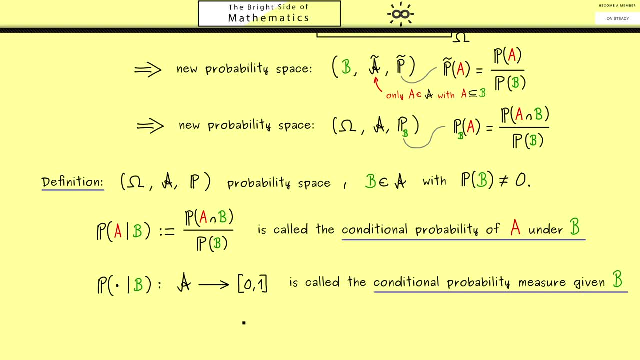 important property, Namely, when you put in b, we get out one. Of course, this is something we get immediately out. Speaking of this definition here, you see, it won't work if p of b would be zero. However, now, sometimes it happens that we simply don't want to check that. Maybe we don't have. 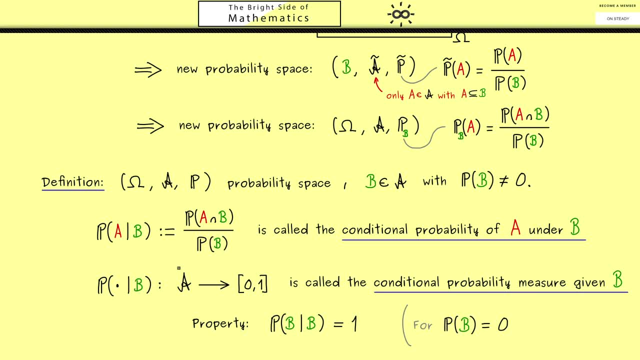 enough information, but we still want to calculate with the conditional probabilities. Therefore, in this case, we will use the following definition: This symbol just represents the number zero, then This will be useful for a lot of formulas later. However, please note here, in this case we don't. 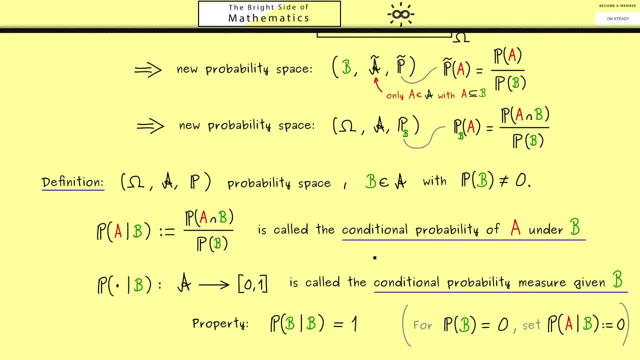 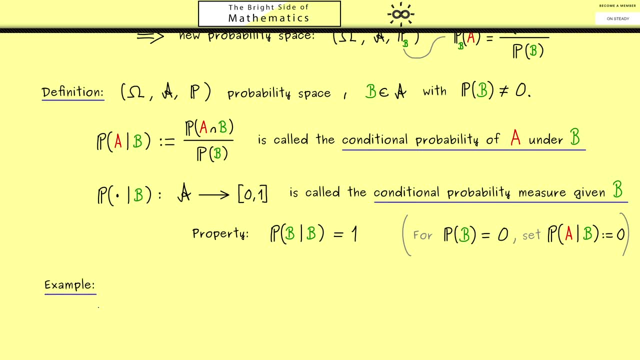 have such a probability measure. Ok, so i think that's enough for the definition. Let's look at an example And, as often, it's helpful to talk about a general urn model. So i would say, let's do something new And look at an ordered one And, to keep it simple, let's consider only four balls with two different. 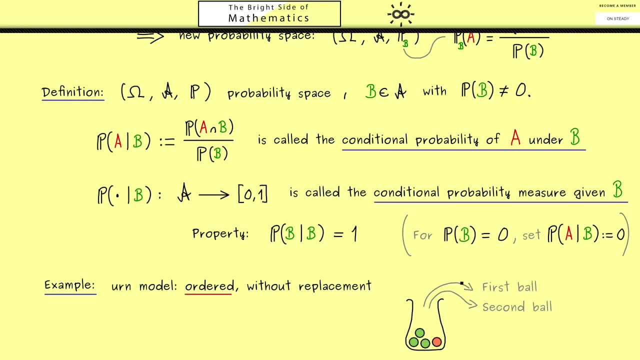 colors, Then let's do two steps: First we take out one ball- We don't replace it, And then we take out the second one. Hence a sample we get is always an ordered pair. It has a first position and also a second position. This means when we introduce a color set c with two colors. 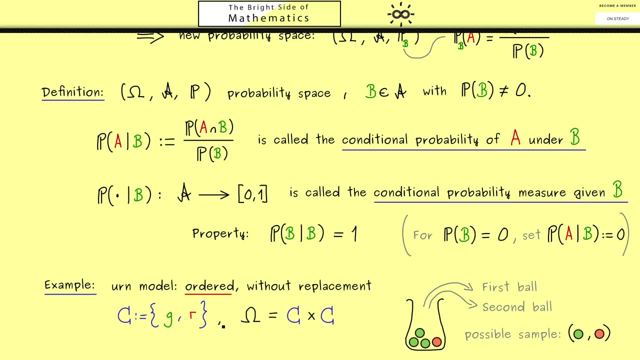 Which is in our case green and red. Then the sample space, omega, is given by the cartesian product of c, with itself Ok, and the sigma algebra, as for all discrete models, is given by the power set. So the only thing missing here would be the probability measure itself. 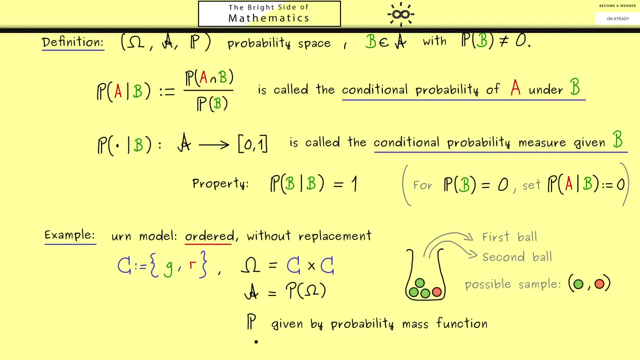 Also here, since we have a discrete model, the probability measure is given by a probability mass function And the best way to calculate this is to look here at the different stages we have in our random experiment. Therefore, i would say a visualization with a tree can really. 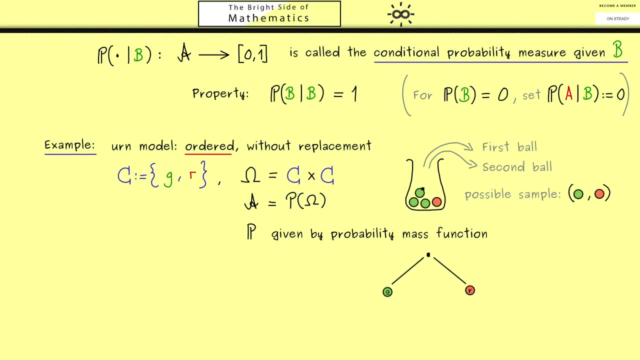 help. So the first stage is very simple: We just take out one ball and the probabilities should be very clear: Three quarters in the favor of green and one quarter in the favor of red. Ok, then in the second stage, we take out the second ball, which also can be either green or red. 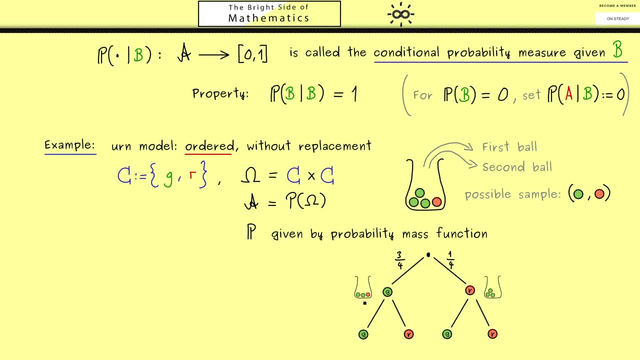 However, now we have different probabilities because we have fewer balls left in the urn. So, for the left hand side, we have two thirds for green and one third for red, Yet on the right hand side, there are no red balls left. therefore, we have one for green and zero for red. Ok then, in summary, with each. 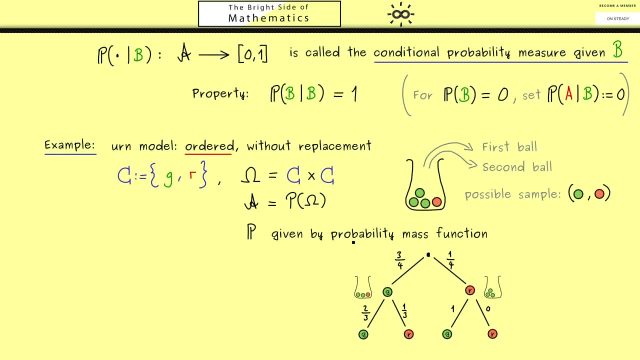 path in the tree. we have exactly one value for the probability mass function. For example, for this path we first have green, then red, so we have three quarters times one third, Which is simply one quarter. On the other hand, first green, then green again gives us one half, Then red, green is also one quarter. 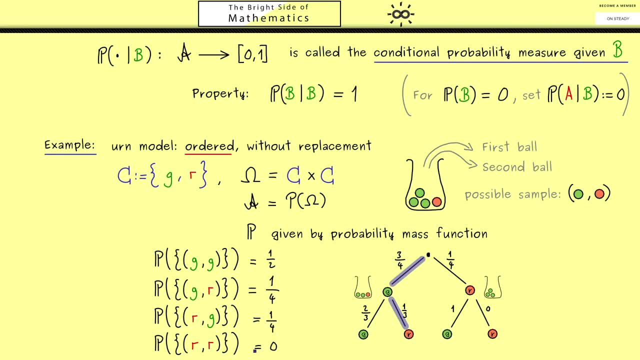 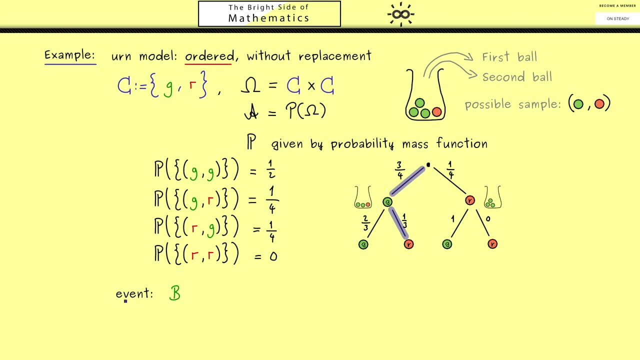 and the other one is zero. Ok, there we have the whole probability measure, and now we can finally talk about the conditional probability. Therefore, let's fix a condition b, so an event from the sigma algebra a. In words, for example, this could be: the first ball is green And in the formula this would: 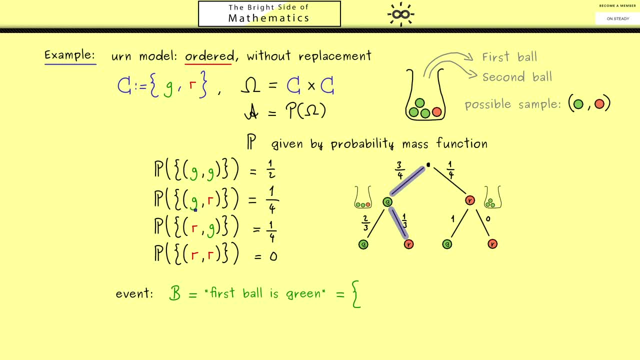 just mean we take the two events that have green at the beginning. So this is our subset of omega we want as a condition. And then let's calculate the probability of gr under the condition b. So this is a nice conditional probability, which shouldn't be so.